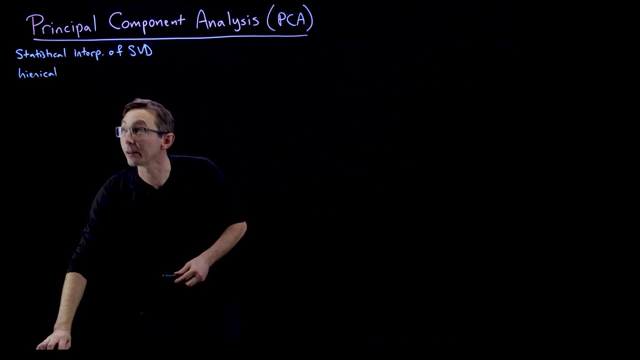 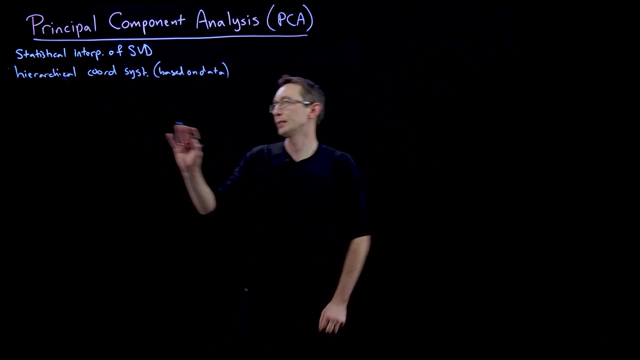 hierarchical- that's not how you spell hierarchical- a hierarchical coordinate system. Hierarchical coordinate system Based on data To represent the statistical variations in your data set. Okay, so it's a coordinate system based in terms of directions in your data that capture the maximum amounts of the variance in your data. 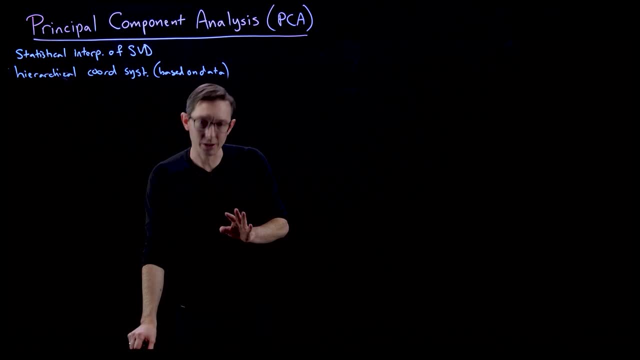 Okay, and so I'm going to. the notation here is going to be a little different than what we're used to, and that's because the PCA literature and the SVD literature, you know, are all very, very, very, very different. So the PCA literature have kind of different conventions about what the matrix looks like. 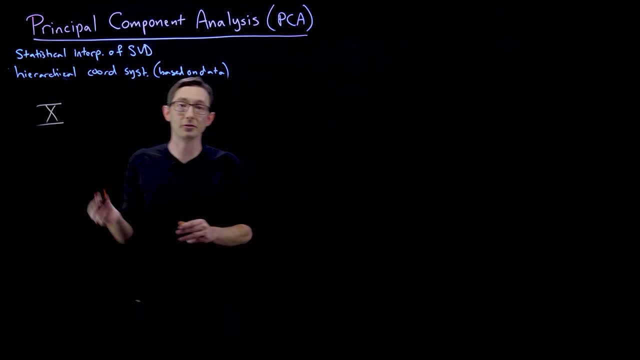 So in the PCA literature we still have a data matrix X and it still has a bunch of measurements from experiments, independent experiments. But here we're going to represent those independent experiments as big row vectors X1, X2, and so on and so forth. Okay, so each row vector X are essentially, you know, 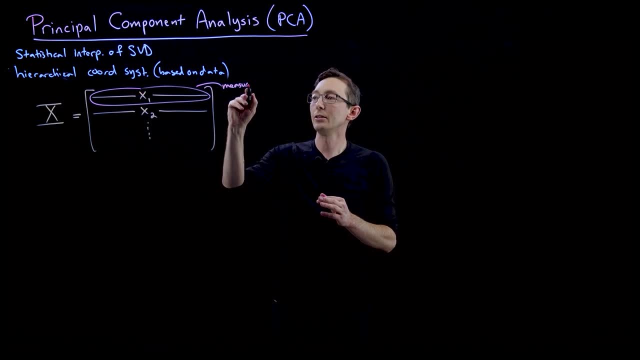 essentially measurements from a single experiment. measurements from a single experiment, and what we're hoping is that these are kind of individual experiments, So this measurement might be the demographic information from a specific human, you know: age, weight, sex, race, et cetera, et cetera, et cetera. 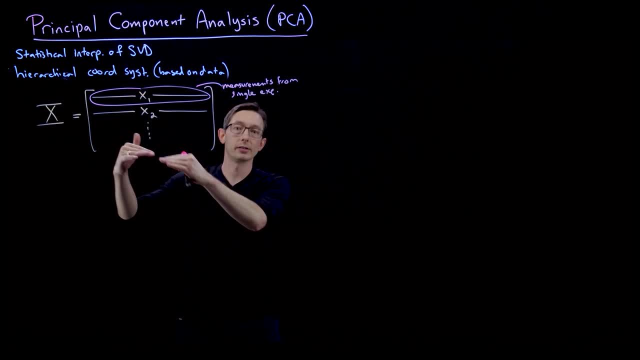 And then X1 would be person one, X2 is person two, and so on and so forth. So the same basic idea as before with our data matrix X, except now, instead of columns having the information for a specific individual- kind of that measurement- from a single experiment- now we're going to have those be rows. 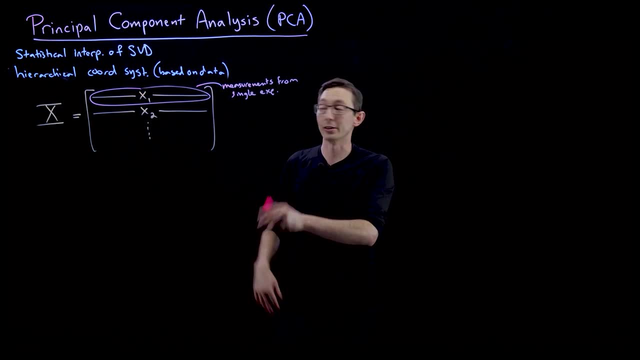 And that's because that's consistent with the PCA literature. So I just want to show you how it looks this way. Okay, And the idea here is that we're going to try to find and we're going to assume that this data X has some 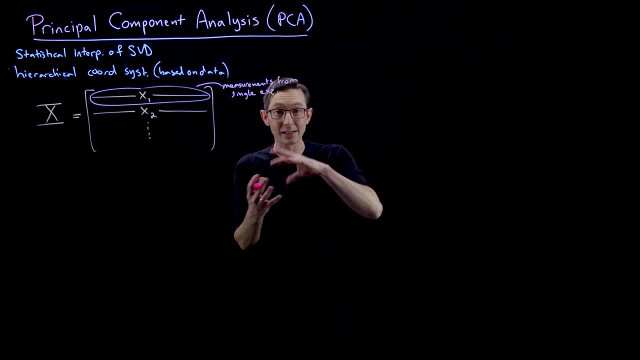 statistical distribution. It's not deterministic. There are some statistical variability. It's not deterministic. There are some statistical variability. It's not deterministic. There are some statistical variability to this information And we're going to try to uncover the dominant kind of combinations of features that describe as much of the data as possible. 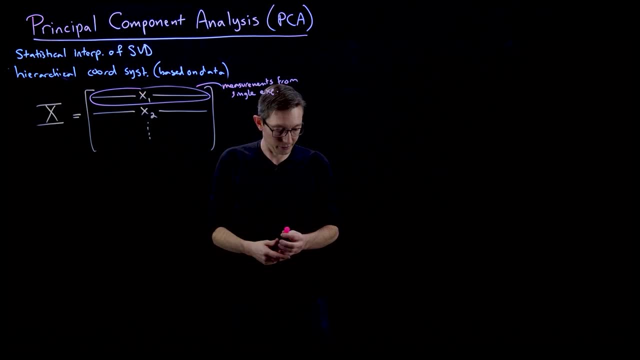 Okay, So we're going to do it using the SVD, but we're going to write it a little bit differently. Okay? So, because this is the statistical interpretation of the SVD, there's a few steps that are extra, that we don't normally do with SVD, that we're going to do here. 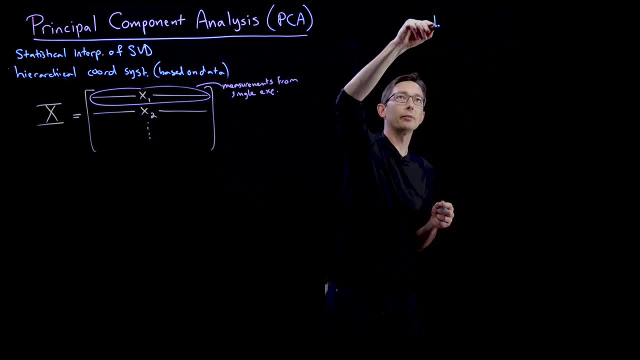 So kind of step one in this procedure is that we're going to combine the data matrix X with the data matrix X, So we're going to compute the mean, the row-wise mean, the average row. So we're going to compute the mean row and we're just going to call this: X bar equals one over. I'm going to say that I still have N rows. 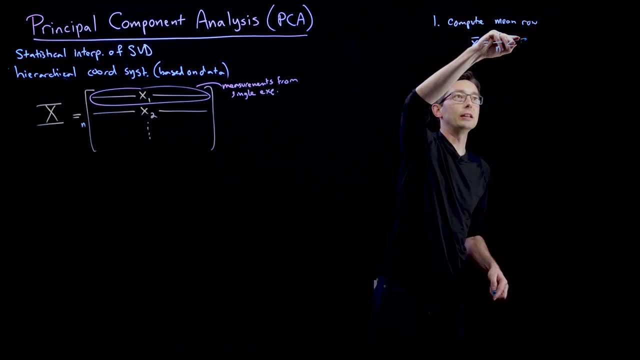 one over N. sum of each of these X Js from J equals one to N. Okay, So this is the average row. I just average all of the rows. The next thing I'm going to do is I'm going to build an average matrix. 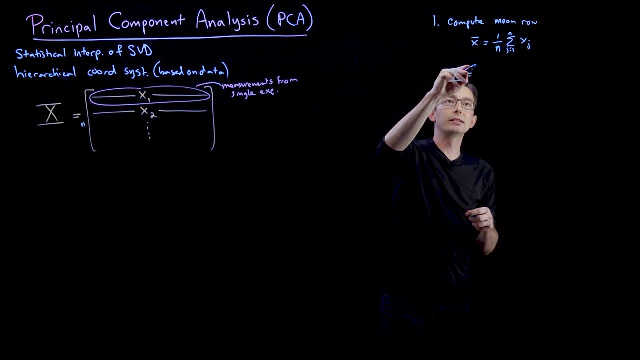 So the average matrix is going to be obtained by taking a vector of ones and multiplying it by that X bar vector. Okay, So I just literally create N copies of X bar, and that's my X bar average matrix. And so step two is I'm going to subtract the mean. 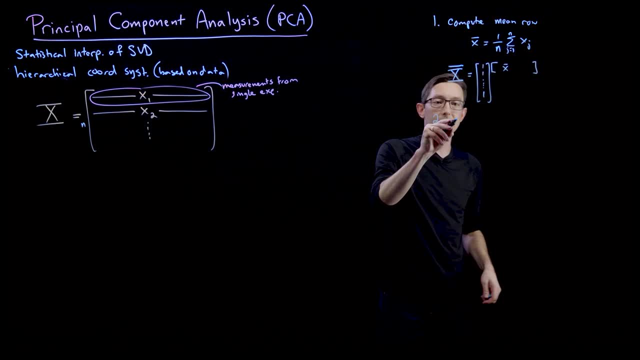 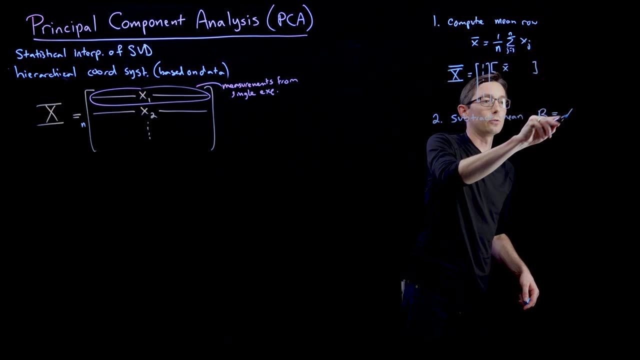 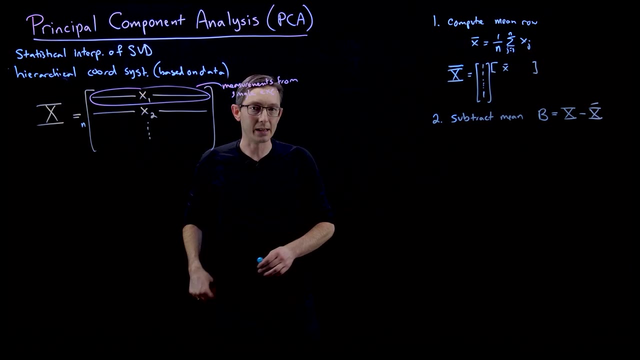 Okay, So I'm going to subtract the mean. So now I have: B equals X minus X bar, And the way we say this in PCA language is that this is the mean centered data. So if I have some distribution of data where there's some, you know, average value to all of this, 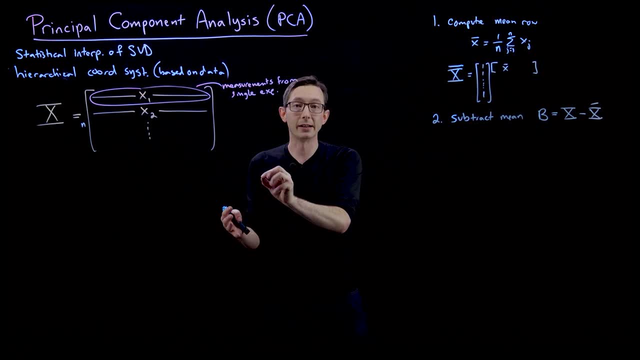 when I subtract that out, it brings everything down so that the center of my distribution is at the origin. Okay, So we're going to be modeling this data matrix X, assuming that it is a zero mean Gaussian, And so this is where we subtract off the mean so that it's zero mean. 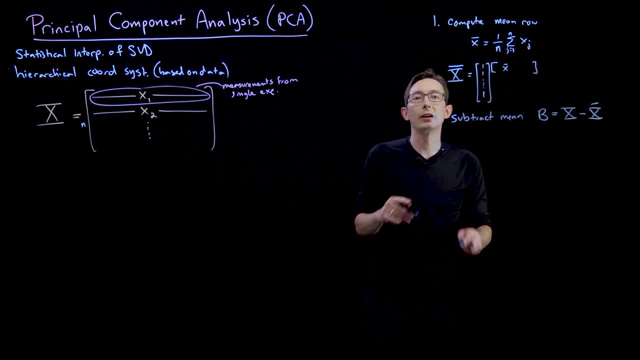 Okay, Now what we're going to do is we're going to compute the covariance matrix of this mean centered data. So the covariance matrix, Again, this is kind of just the correlation matrix from the end. This is the correlation matrix from the SVD. 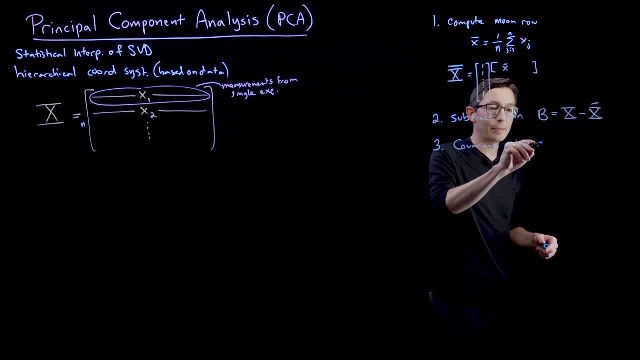 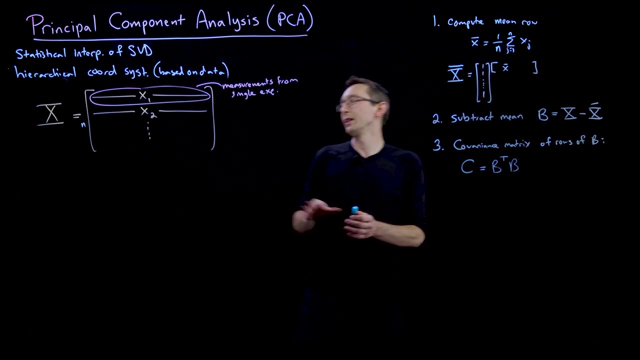 But we're calling it a covariance matrix in this context. So the covariance matrix of the rows of B, And we're going to call that matrix C, C is equal to B. transpose B. Okay, Good. So at this point all we've done is essentially take our data matrix. 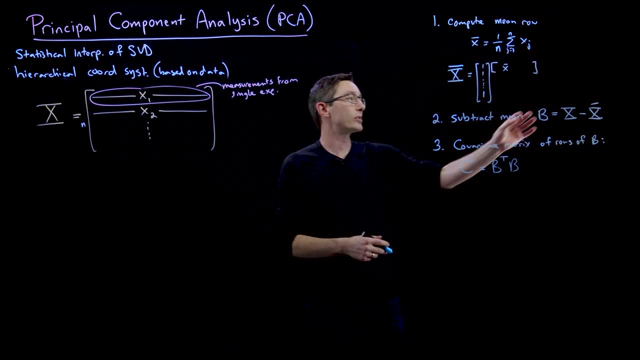 We've written it in a transpose from how we normally do it. We've subtracted off the mean And we've computed this correlation matrix or this covariance matrix. So this looks a lot like the X transpose X from before, but we've subtracted off the mean. 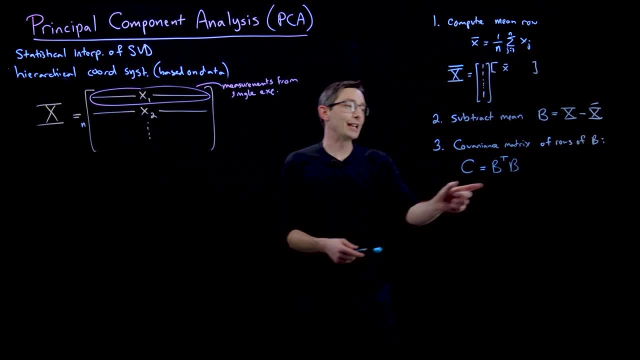 Now, what we're going to do is we're going to compute the eigenvectors, the leading eigenvectors of this correlation matrix, And that's going to be related both to the singular vectors of X and also to its principal components. Okay, 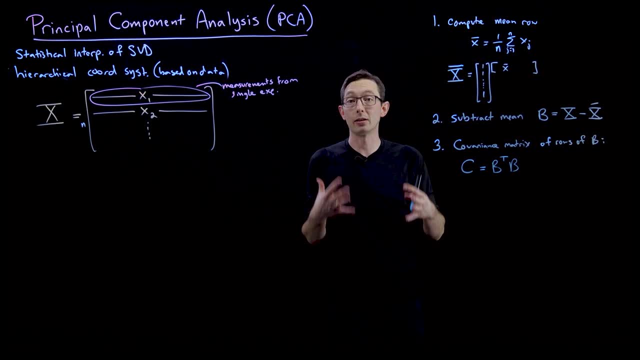 And I'm going to try my best to get the notation and the terminology correct. Again, this is in section 1.5.. So you can go there to refer for more details. Good, So now what we're going to do is we're going to compute the eigendecomposition. 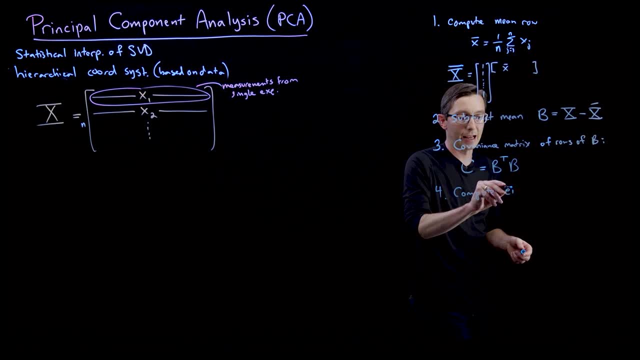 We're going to compute the eigenvalues and eigenvectors, So the eigs of C, And in particular, we're going to compute, for example, let's call it: V1- transpose B, transpose X. Okay, V1, transpose B, transpose B, V1.. 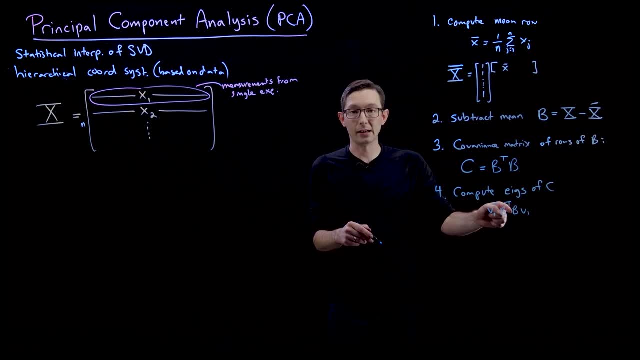 That would be the biggest eigenvector of this matrix. B transpose B is V1. Then I would compute V2, then V3, then V4, and so on and so forth, Just like in the SVD. And there's corresponding eigenvalues, just like in the SVD. 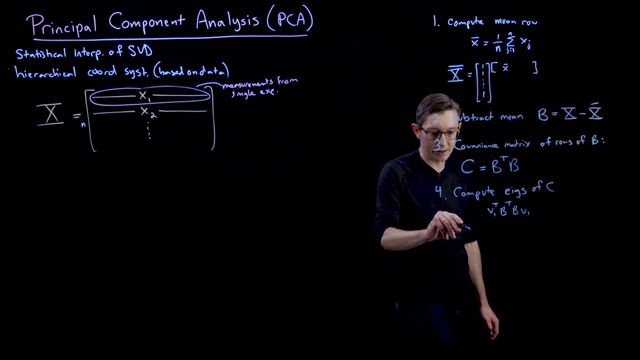 And essentially what we're going to get is this matrix: C times V equals V times D, Where these are my eigenvalues And these are my eigenvectors. Okay, Good, So all we've done is we've computed the singular, sorry, the eigenvalue decomposition of this covariance matrix. 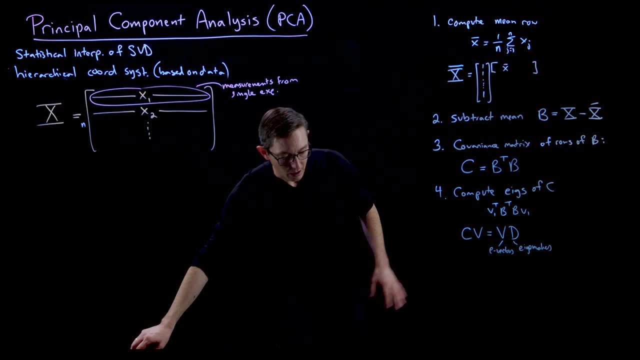 Now you could actually compute it using the SVD- I'll show you that in a minute- And you get these eigenvalues and eigenvectors, And here's where the principal components come in. So if I take this matrix T, which is equal to my mean subtracted data B, 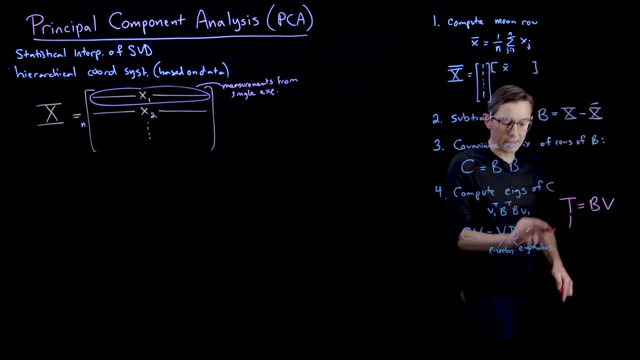 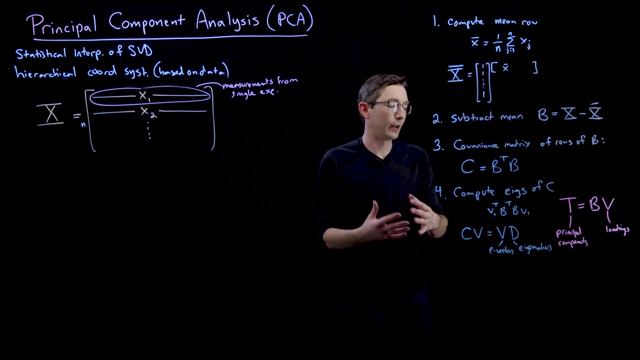 times these eigenvectors V. these are called my principal components. These are my principal components- Okay, Principal components. And this vector V of these eigenvectors are called the loadings. So essentially what you do is you decompose this matrix into kind of directions of maximal variance. 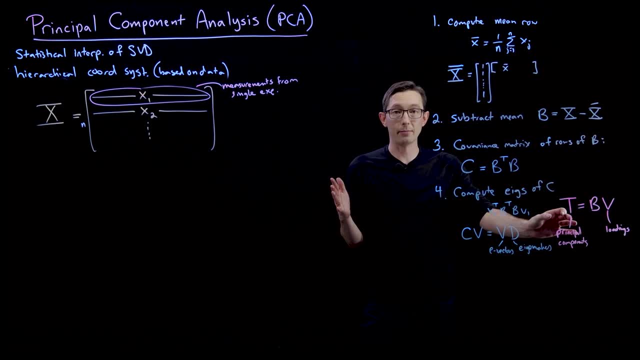 Just like in the singular value decomposition, Called the principal components And the loadings are kind of how much of each of those principal components each of the experiments has The loadings in a particular experiment of those principal component columns. Okay, And oftentimes in terms of the singular value decomposition language. 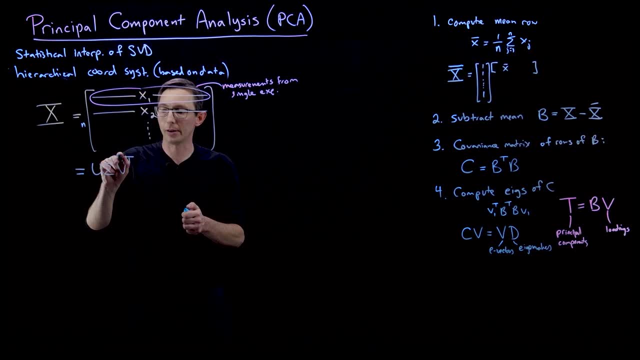 so let's say X was equal to U sigma V. transpose here, Then what we would say is that T is simply simply equal to U times sigma. Okay, Because- and if I write B as sorry, I should be a little bit more careful. 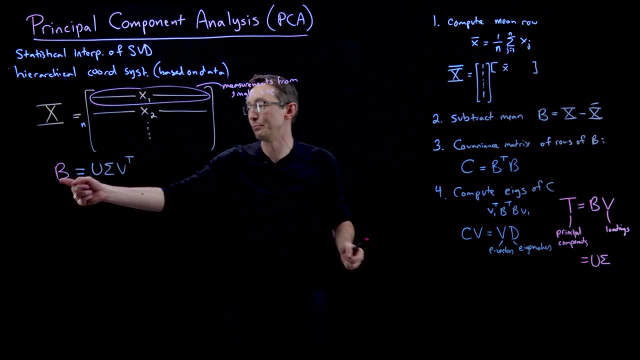 If I took the singular value decomposition of the mean subtracted data, B equals U sigma V transpose, Then T would be either B times V And B times V is simply U times sigma. Okay, So that's a representation of the principal components. 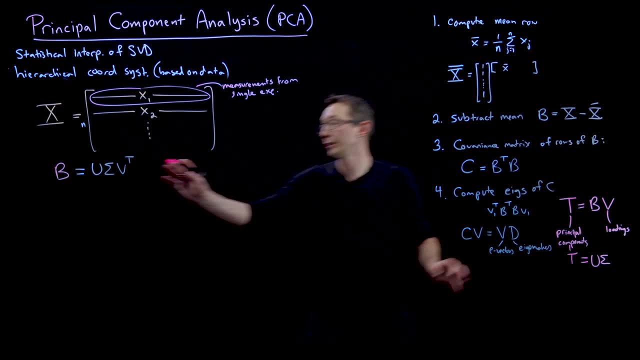 Okay, So you can get the principal components and the loadings directly from the SVD of the mean subtracted data. I guess that's the headline here Is that this very important statistical representation of your data can be achieved just by computing the SVD of your mean subtracted data. 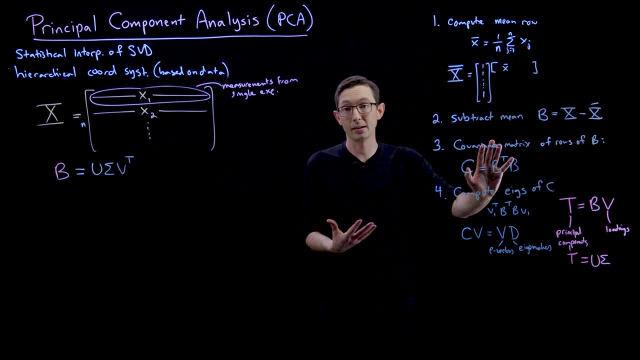 It's the same as finding these eigenvectors of the covariance matrix, Which is what you would kind of do in the classical principal component analysis. Good, Okay, Now what's also important is these eigenvalues here, or the singular values in sigma. 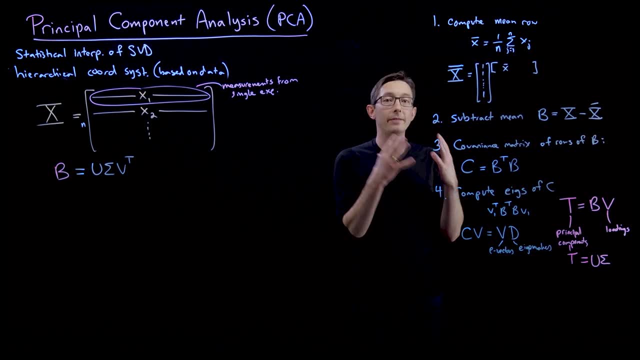 give you an indication of the amount of the variance of this data set that these principal components capture or these loadings capture. So if I only want to describe this high dimensional data in terms of the first two principal components and the first two vectors of loadings, 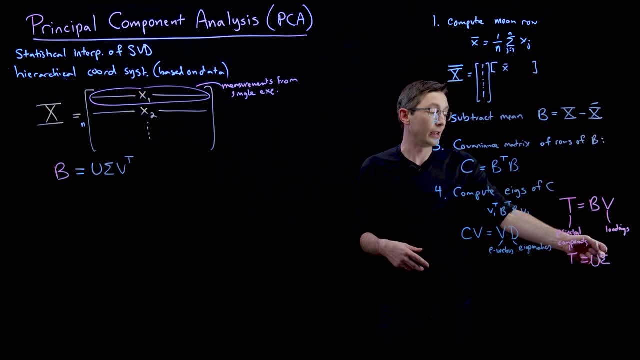 I would be able to compute how much of the variance is captured by computing, kind of how much energy or variance is in those first two eigenvalues of this D matrix, And so what I could literally do. I want to make sure I'm being careful here. 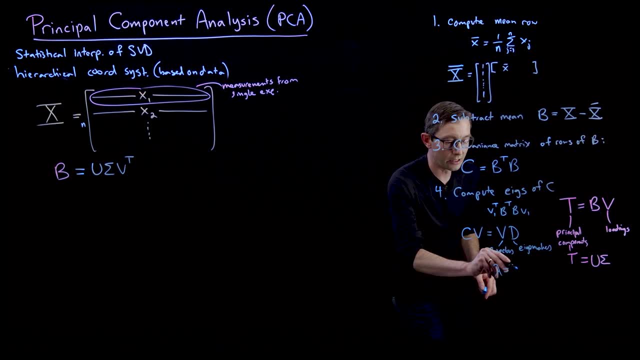 these eigenvalues lambda are equal to the square of the singular values, and it's literally equal to the variance of that principal component in the data. And so if I want to know how much variance is being captured in the first, let's say, R, mode, 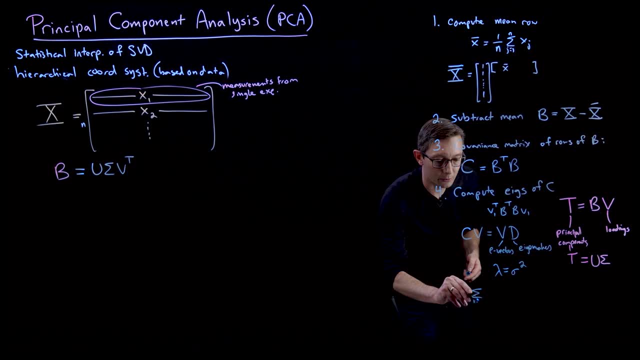 I would take the sum from k equals one to R- of lambda k divided by the sum of all n of my lambdas. So I would basically see what's the fraction of variance captured by my first R lambdas divided by the total of all of my eigenvalues. 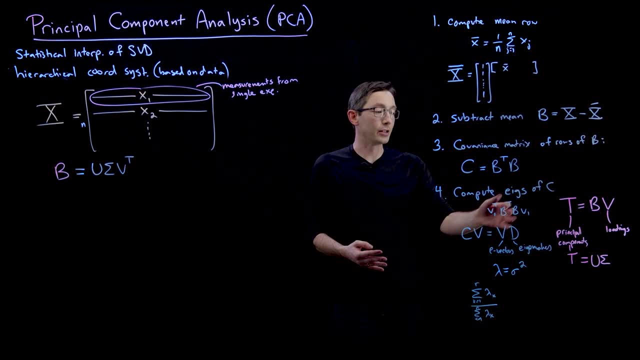 all of the variance in the data, And so, for example, I might decide to keep only as many principal components as are needed to explain 95% of the variance, And so that would give you a criterion for how many principal components to keep. 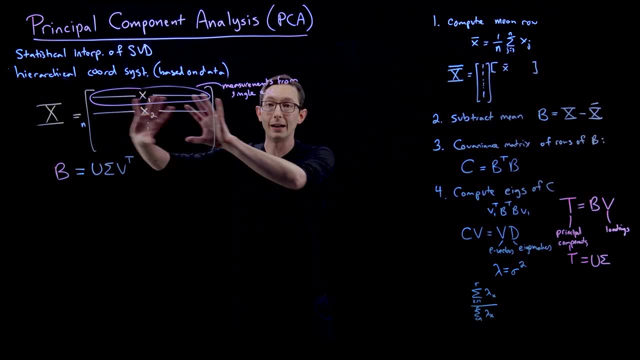 Okay, again, we're going to code this up. I'm actually going to create a couple of data matrices, real data matrices that have distributions. One of them will be a random data matrix. Another one will be a data matrix consisting of genetic markers. 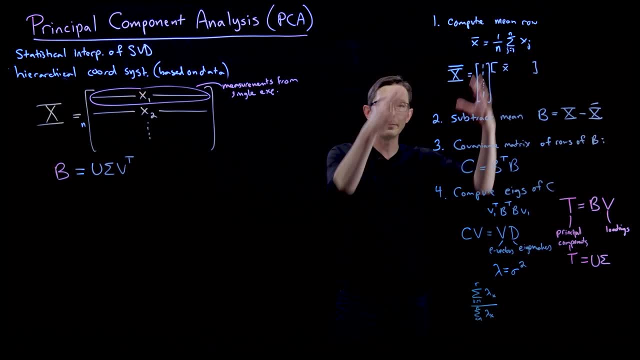 for people with and without ovarian cancer, And we'll compute this principal component analysis and look at the results. So I'll point out that, again, in MATLAB it's pretty easy to compute this. So it's something very simple, like V score. 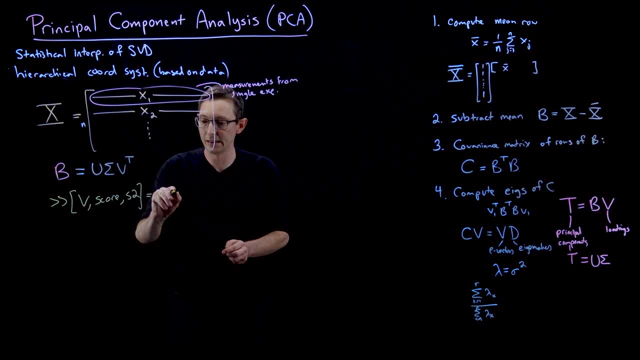 and then some extra variable: S2 equals PCA of the B matrix. Okay, so really really easy to compute in MATLAB, also easy to compute in R and Python, and so we'll do examples of that. The last thing I want to do is just show you a picture.